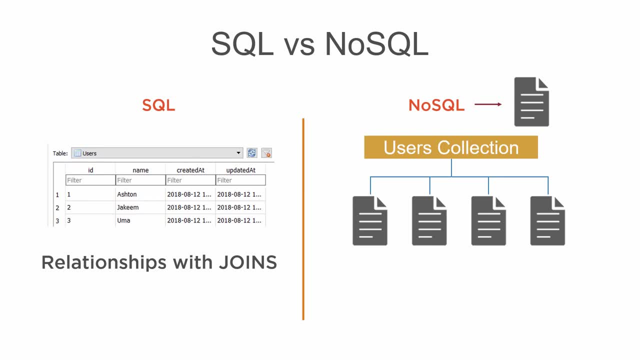 We might have a collection of users, with a document for each user containing specific user data, such as name and email. One way to organize our data is by creating sub collections So, for example, for every user document that's created, that user may also have a sub collection of books. 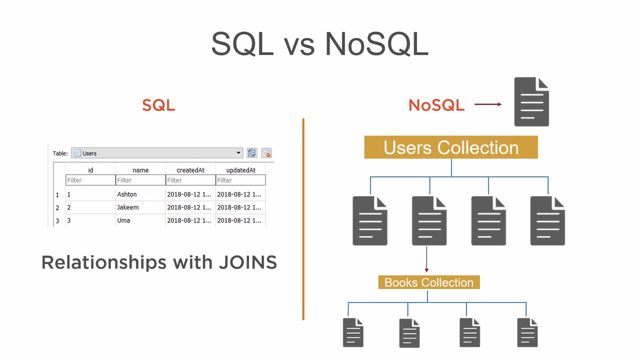 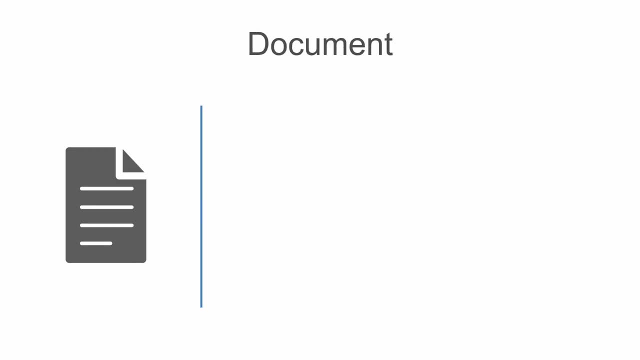 with the data for each book stored inside of a document. Now let's talk about what these documents look like. Documents store its data in key-value pairs, just like an object. Every comp combination of key and value pairs is known as a field, So inside of Firestore, when saving data. 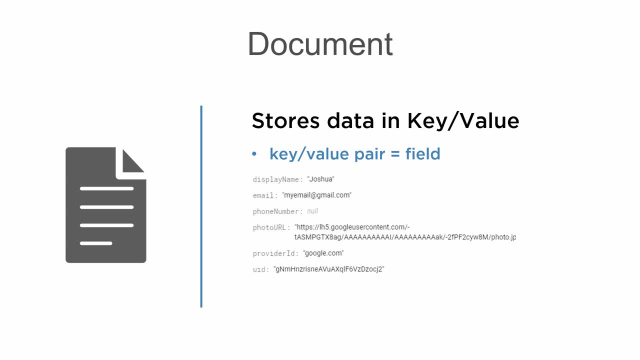 for a user using Google authentication. the result would look something like this: Each key within a document represents a static name for an entry. The value can be any type of data that you're probably already familiar with, such as strings, integers and booleans, Because the type of data 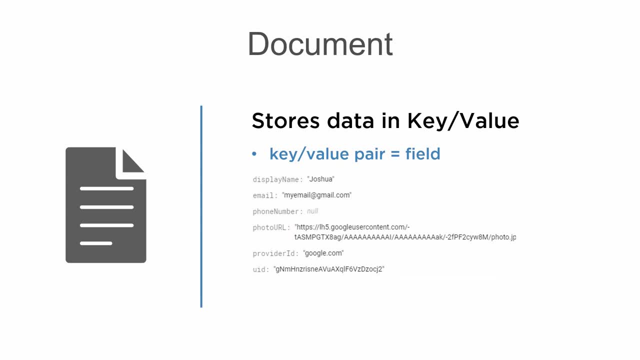 saved to each field is not strictly defined. it is a very good idea to make sure that we are defining our field types inside of an interface in our Angular front end.